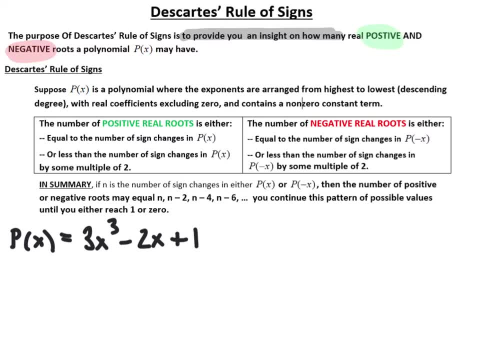 Now what it says. listen to this. it's kind of cool, is? it says that the number of positive real roots is either equal to the number of sign changes that exist in that polynomial, or the number of sign changes minus a multiple of 2.. 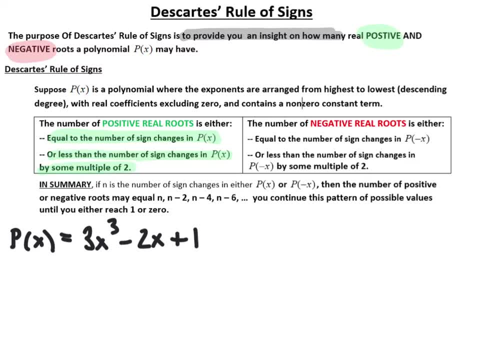 Let me explain. Let's look at the one I did here. So the first term has a plus as its sign, then a minus and then a plus. So how many times does the sign change? Once, twice. What this means is there were two sign changes, so the number of positive solutions there could be could be 2 or 0, because again, we can subtract a multiple of 2 from it. 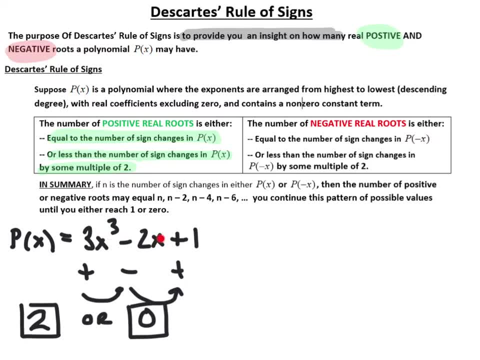 So when you and I solve this problem there, we can expect either to have 2 positive answers out of the 3, or no positive answers out of the 3.. Now this also can tell us about the negatives. Let's see what it says. 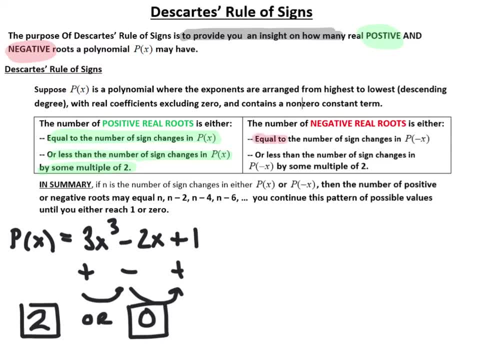 It says the number of negative roots is equal to the number of sign changes in P where we put in minus x Or that amount less by a multiple of 2.. So let's plug in P of negative x. So when we put in a negative x into the original P that would be 3 times negative x all cubed minus 2 times negative x plus 1.. 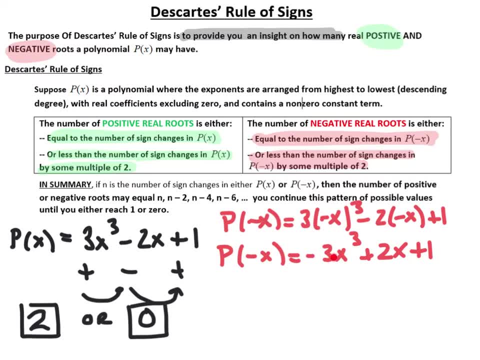 When we simplify this, the first term then becomes negative, 3x cubed, This becomes a positive 2x and a plus 1.. Now, when we assess how many times the sign changes, it changes once here, and that's it. 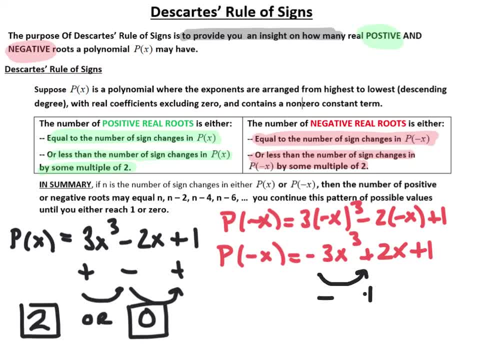 Because it went from negative. it went from a negative to a positive and then it stayed positive- one switch. So actually this informs us in this case that there will be one negative solution. So we learn quite a bit by plugging in this information and determining what we get. 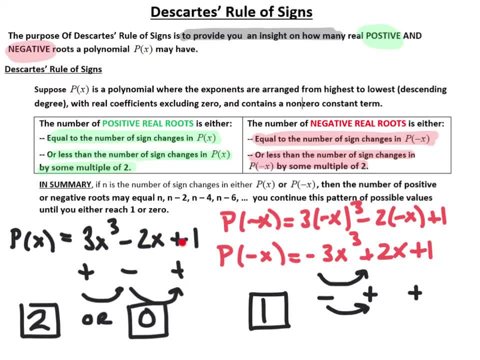 Either the positives are how many sign changes there are, or that value minus 2, or minus 2 down to 0 or 1.. Here the same thing happens. here We would find how many sign changes take place in P of negative x. 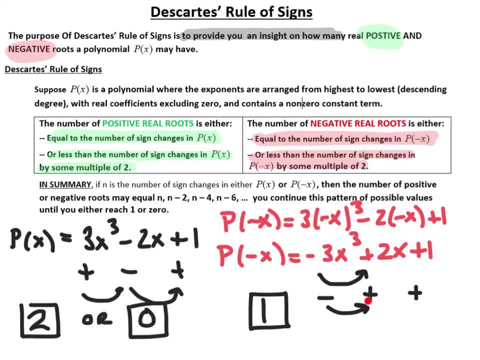 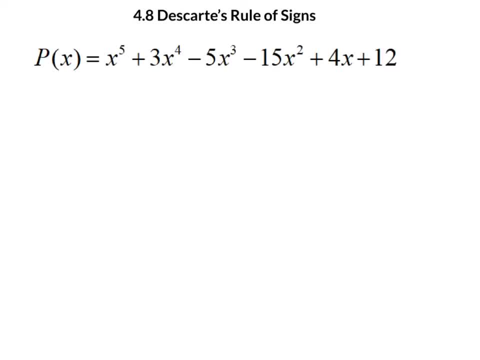 And then again, if this was a higher number, we would do the multiples less by 2. But in this case there was only 1.. Let me do a bunch of examples and more of it will come clear. Let's see how many times a sign changes. 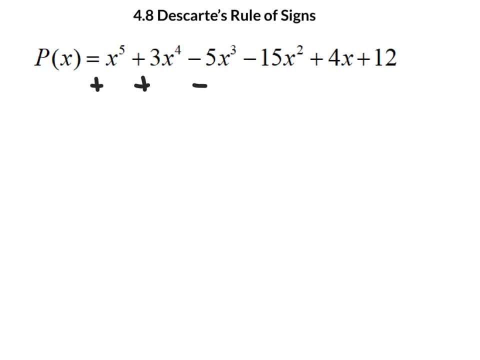 Maybe it's easier if I just mark the signs out for a minute, So let's do that. So when did the sign change? Here it changed, And here it changed Right- Only twice. Do you kind of see how that works? 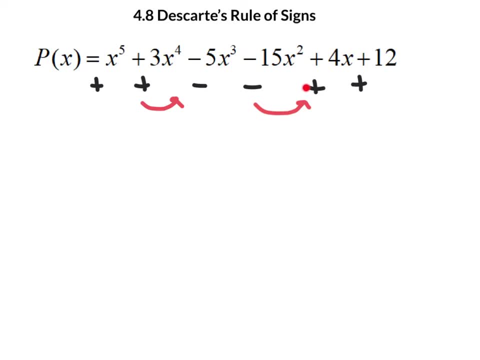 So the same change, same change, same, So 2.. So our answer to how many positive answers of the 5 we can expect would be 2. Or 0.. Next let's look at the negative possibilities. 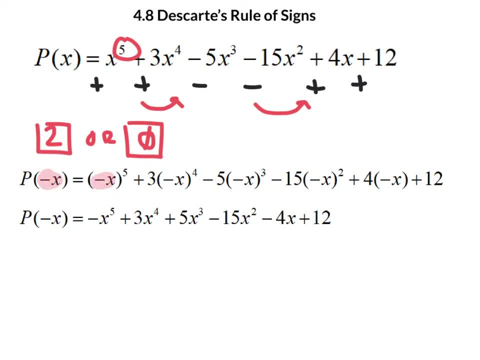 So to look at the negative possibilities, I plug in negative x wherever there's an x throughout that term and then just simplify to keep an eye on the signs. So let's do like we just did after we've simplified that. 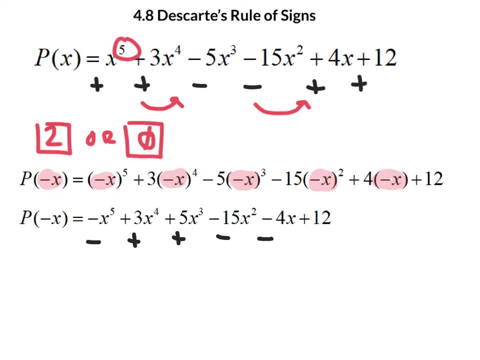 That goes: negative, positive, positive, negative, negative, positive. And we will look for how many times we get negative x And we will look for how many times it changes: Once, twice, three times. So actually that means this guy could be 3.. 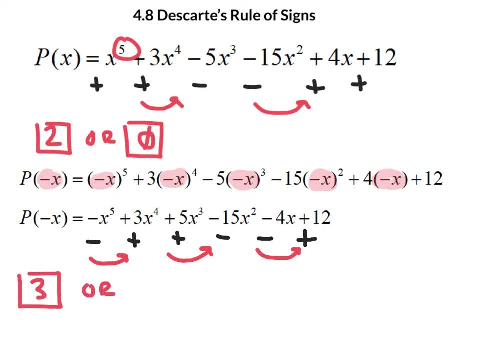 There could be 3 negatives Or there could be 1 negative. So this is what the law Descartes' Law of Science, really tells us: Is that in this case, out of the 5, it could be 2 or 0, or 3 or 1.. 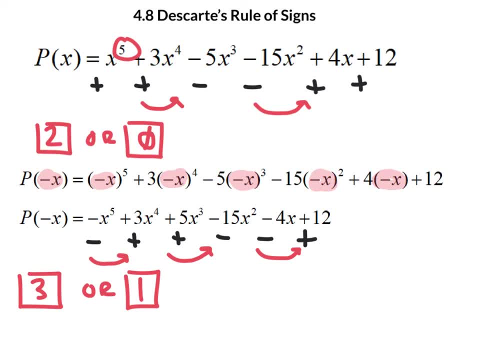 Now, if we put this all together in a chart, we can see even more information. Now, if we put this all together in a chart, we can see even more information. Let's put all of this just up in a corner for a minute. 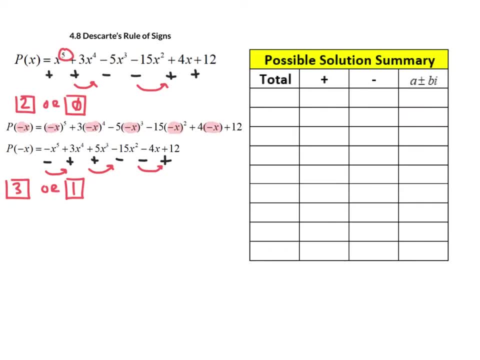 All right, let's see how this all comes together. We know that there are 5 solutions to this, And I'll just put the number 5 down. a bunch of these, because that won't change. Now. from this information right here, we know that you're either going to have 2 or 0.. 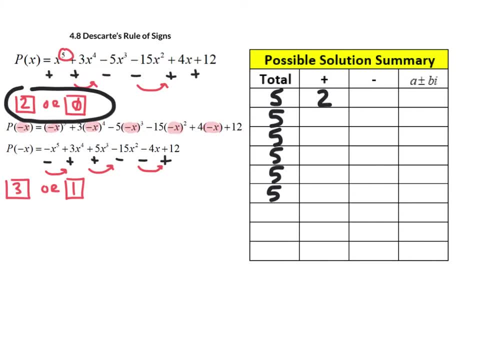 So let's start with the idea that there are 2.. If there are 2 of those, If there are 2 of those, what would be left over in terms of the negatives? So there are 3 remaining right. 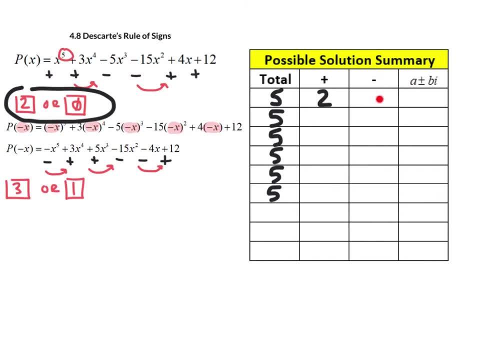 If I started with 5, I have 2.. There's 3 more values that could go here, And we learn that there could be 3 that are negative, And so we could put in our 3, and that would mean there's none of those. 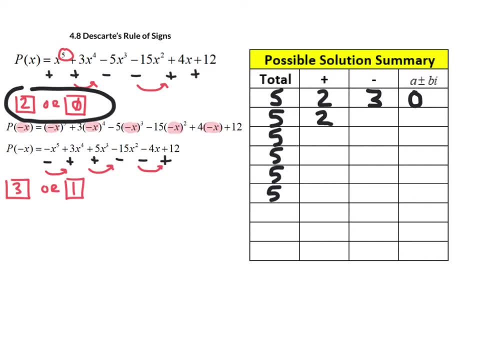 Let's keep our positive the same. There could be 2 positive, But there also could be just 1 of those. So let's say, oh, maybe there's just 1 negative. That would mean the other answers had to be complex. 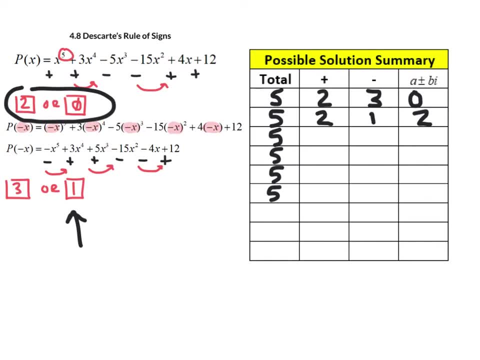 So what I'm doing here is I'm listing out all of the things that could happen, And the way I do it is I lock in like the first positive, So I say: all right, what are all the things that, when you had 2 positives, 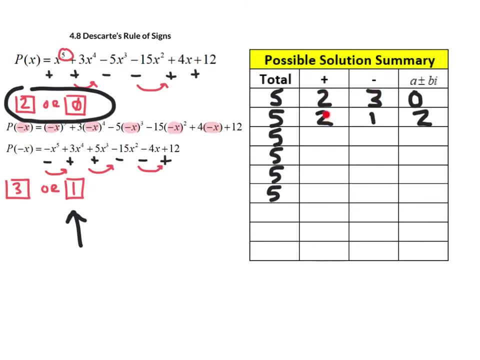 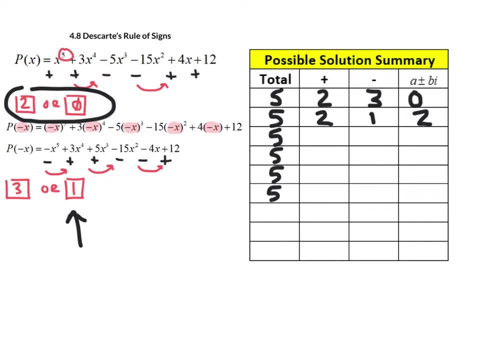 Now I go back and I say: well, what happens if you had 0 positives? So if I had 0 positives, that would mean at most I could have 3 negatives. But I still need 2 more answers, because there are 5 in total. 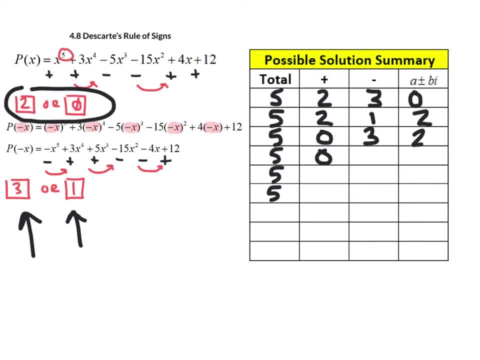 So that meant that there would be 2 of those. What happens, though, is if I didn't get the 3 over here, but I got the 1. And so that would mean I would have 1 negative, and that would mean there would have to be 4 of those. 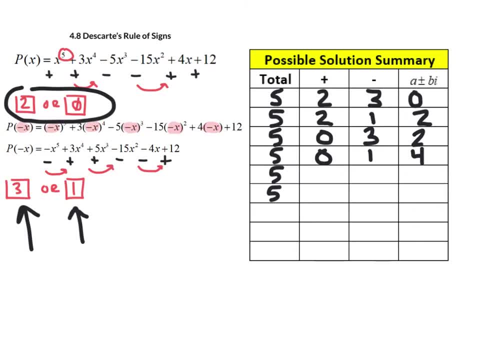 Now I know that the first time you do this it's a little tricky, And what I do is I kind of just keep all of the positives. I do all of the things that could happen with that first positive. What are all the things that could happen? 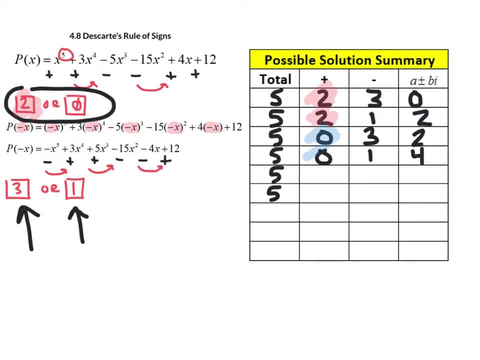 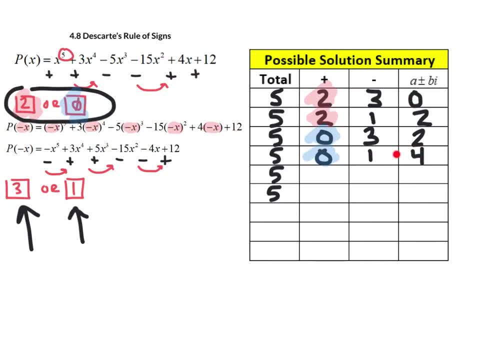 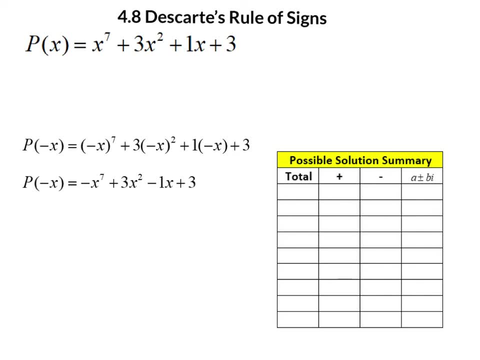 These are the 4 combinations of what could happen in this particular problem. Let's do another example. Let's see how many times the sign changes in this case. So it's positive, then it's positive, then it's positive, then it's positive. 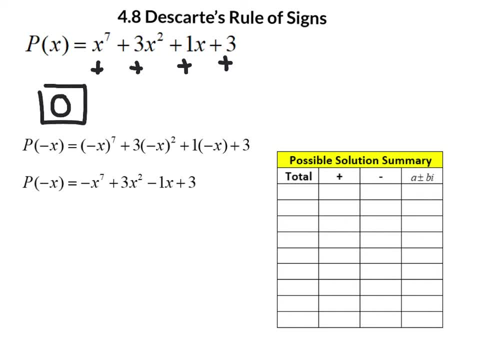 Whoa Zero. There will be no. there will be zero positive answers. If the sign never changes, then there won't be any positives. Let's go to our negative situation. So if we plug in the negative into each of those, 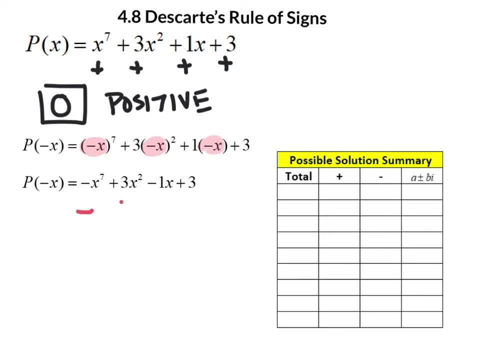 it eventually simplifies and it goes: negative, positive, negative, positive. How many times does that sign change? Once, twice, three times. So in this case they'll either be 3 or 1.. So again, how do I handle that? as to all of the things that could happen, 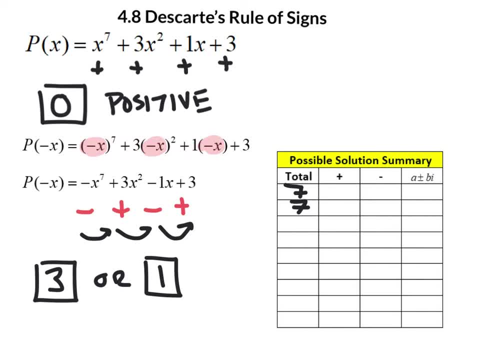 Well, there are 7 answers. Whoa, That's a lot. So I just always just put a bunch down here: 7. Now this tells us there will always be zero positives. All right, So there's no change in that number. 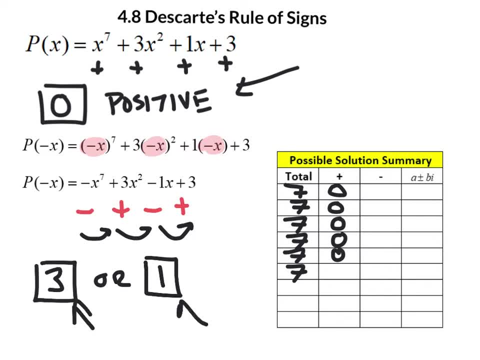 And you either have a 3. Or a 1.. So let's try the 3 first. That would mean that there would be 4 imaginary answers, Or you could have 1 negative and you would have 6. Actually, that's all there is. 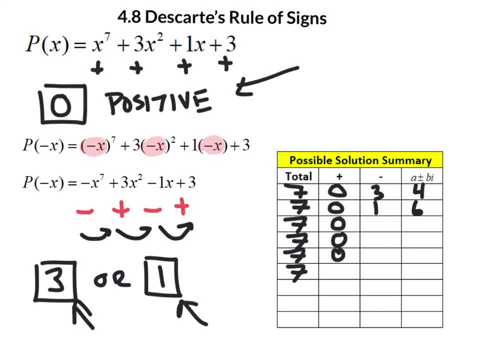 There are no more different options here, because this doesn't change at all, And you're either a 3,, and that would mean 4 of those, Or you're a 1,, which would mean 6 of those. So these are the only two things that could happen to us, using Descartes' Rule of Sines. 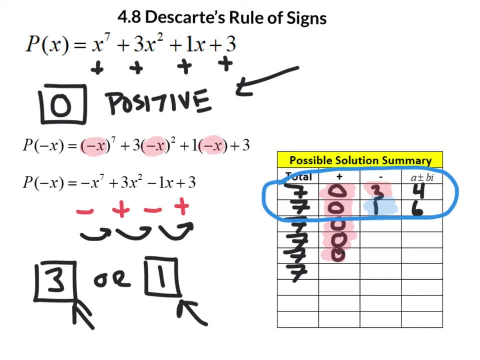 You're either going to have 3 negatives and 4 complex answers, Or you're going to have 1 negative answer and 6 complex answers. You'll not get any positive values to this guy. Let's do another one. Let's save some time. 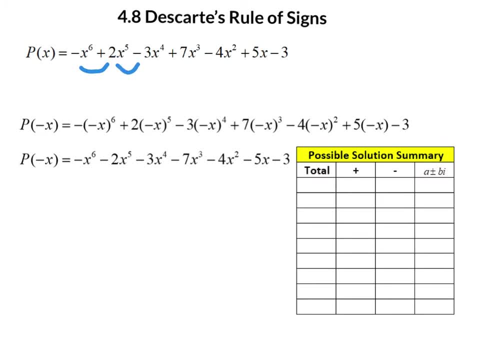 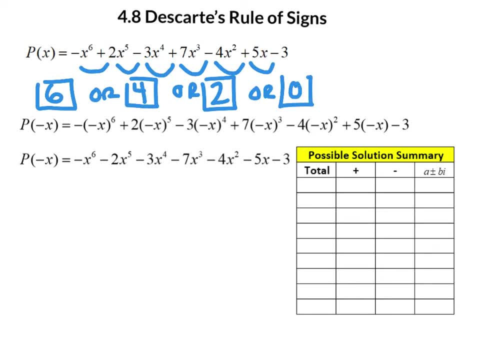 Or 1. 0,. I mean Sorry, Now let's go check out when we plug in the negative into each of those right along the way, And we simplified, How many changes do we see? Hey, wait a minute. 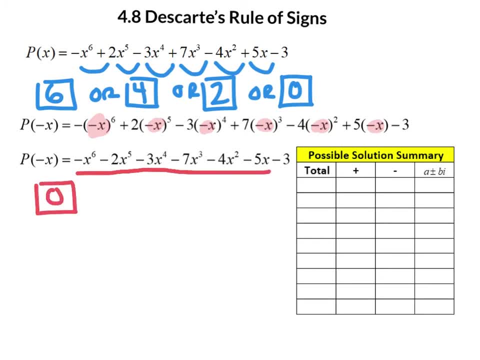 There are no changes, So there's going to be 0 of these guys. Oh, So how many solutions? Ah, there are 6.. Let's fill in our little chart So we know there's always going to be 6 answers. 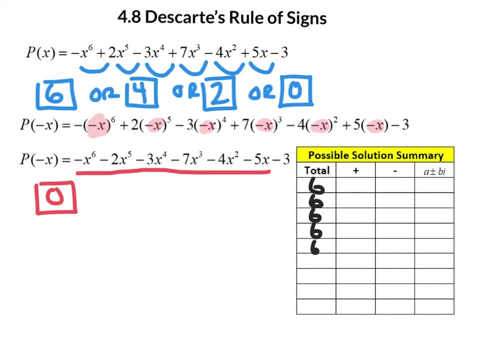 I'll just put a few 6s down here, And all 6 could be positive. none, Actually. we know these are always going to be 0s, don't we? Because there aren't going to be any. So again, that would mean 0 complex. 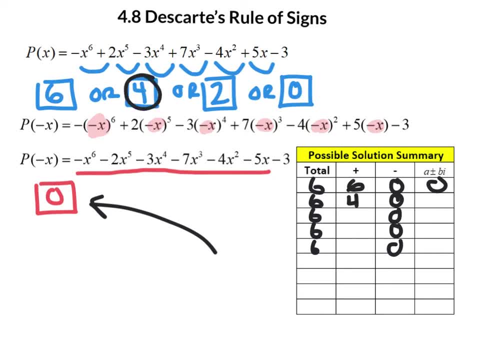 Well, we could have got 4.. We could have got 4 of these, which would mean 2 complex. We could have got 2,, which means 4 complex. Or maybe we got 0 positive and we would have got 6.. 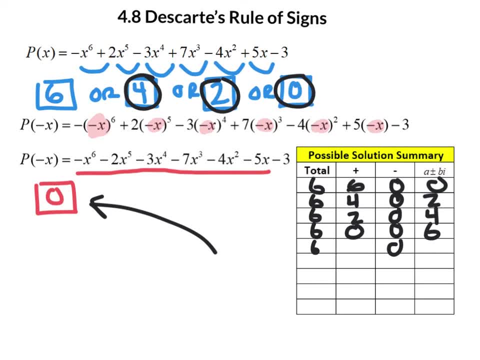 So actually these become our options. You could have 6 positive and no negative and 0 of those. You might have 4 positive and 2 complex, 2 positive and 4 complex, Or 0 and 6.. And that group? 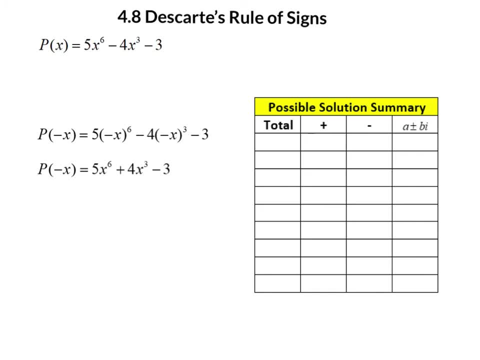 One last example. Let's take a look at our sign changes. So we did a sign change here And that's it So. positives, they'll just be one of them, for sure There's one. And then when we plug in our negative there we actually only see one sign change. 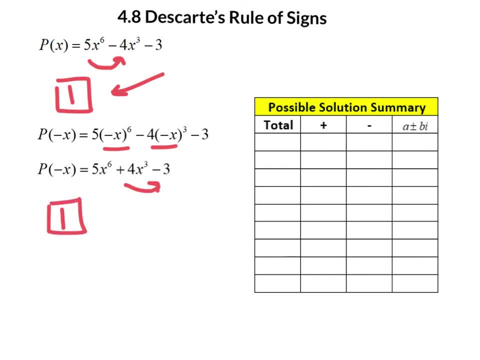 So there's one of these as well. So actually this is pretty simple, because we know that there are 6 answers. One will be positive, one will be negative, which guarantees that the other 4 have to be here, And that's it. 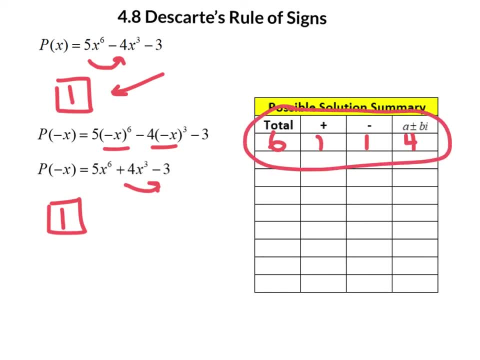 This is what we know using Descartes' rule of science, Because there is one positive and there will be one negative, And so the other 4 have to be complex. Let's put it all together. Alright, here's some giant. 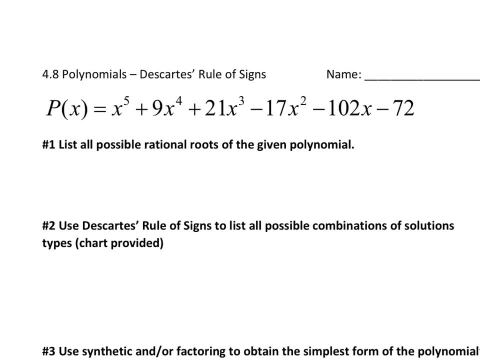 It is giant polynomial And I'm going to break it all the way down to itself Small pieces. So first of all, they ask me to list the rational roots, which is the 72 factors divided by the 1 factors. There are a lot of factors. 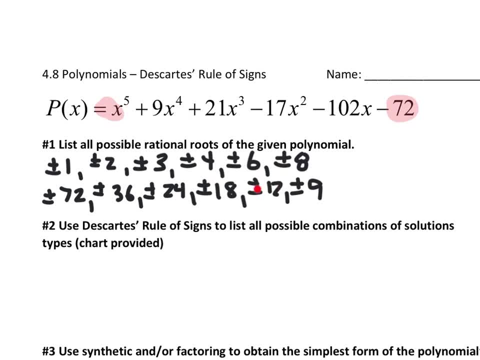 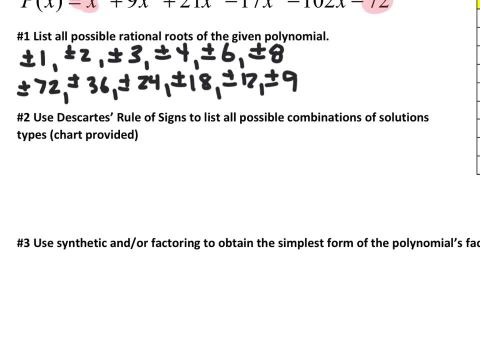 So to some degree we're just there's. where do we start? right? But let's go to the next thing. It says: use Descartes' rule of signs to list all of the possible combinations. So let's do that next. 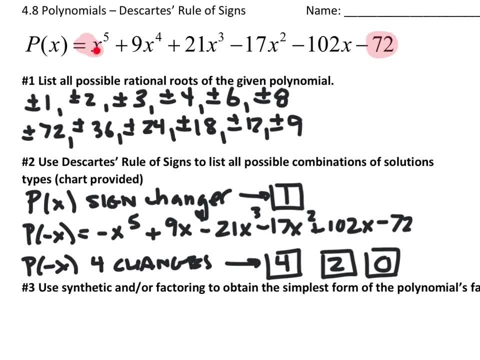 So the first thing we want to do is look at our sign changes. We notice positive, Positive, positive, positive- One sign change. So P of X actually only has one sign change, which tells us there is exactly one positive answer. 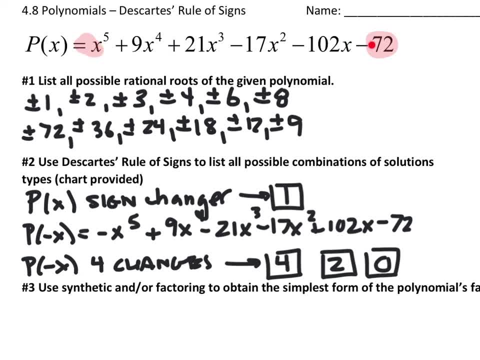 Next I plug in the negative X into there And this is what comes out as P of negative X. I notice it changes once, twice, three times, four times. That means there are 4 negative or 2 negative or 0 negative. 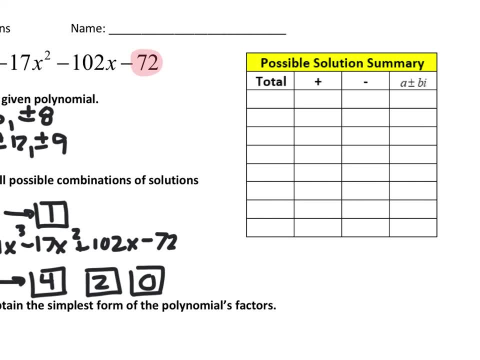 Let's fill out our chart. then There is a total of 5 answers and we know one of them is positive, So I'll fill out a couple of rows of that. Now we learn that there could be 4 negative. 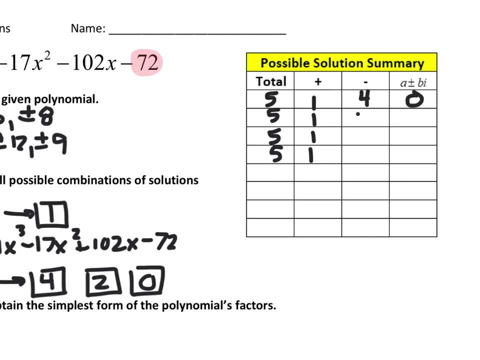 That would be enough to fill that up. Or there could be 2 negative, which would mean there would be 2 of those, Or there could be 0 negative, which would mean there would be 4 of those. These are actually the only three things that could happen. 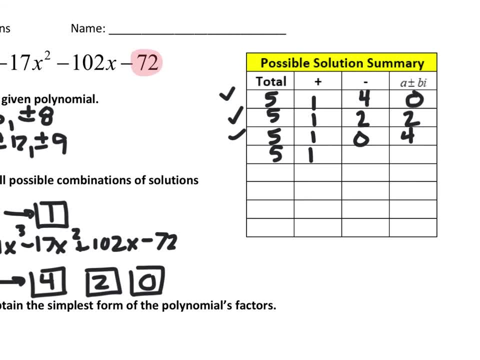 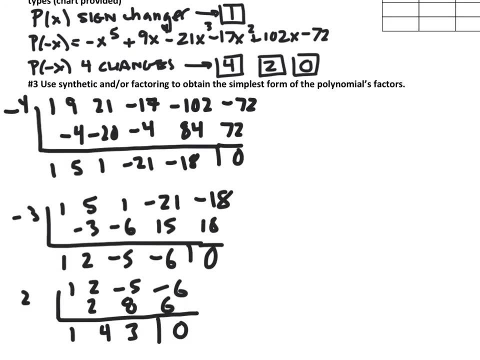 And we'll see which one, But we do know that there will be one positive, and there could be 4,, 2, or 0 of these. Let's keep building our knowledge. Alright, I've done the work here, just to speed us up a little bit. 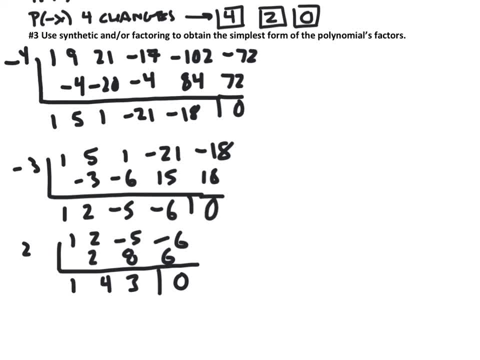 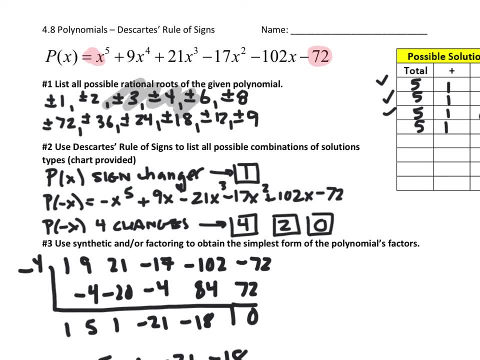 But, as you know, I'm going to pick different values off of my list up here. I'm going to start down in this range just because I've got to get it right. I'm going to start down in this range just because I've got to get it right. 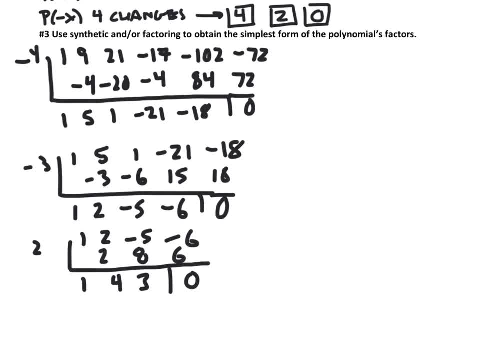 I'm going to start down in this range, just because I've got to get it right. So I begin the process Now. when you do this, of course, you don't always get lucky to make it work. I've picked the ones that will work, just so you know. 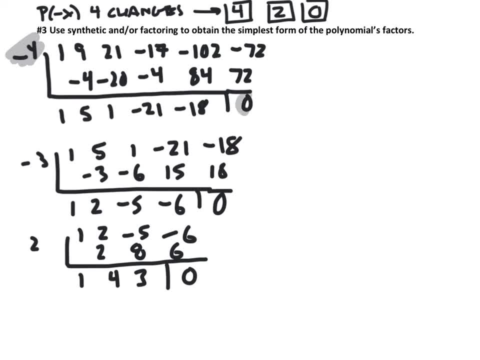 So I picked a negative 4.. I worked my way through it and I got a 0.. What I then do is I have a new factor right here, And it's again not easy for me to factor it my normal way. 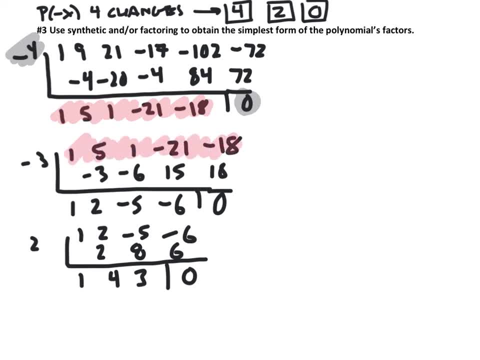 So I throw that value directly back into synthetic division and I take a new shot at it with a new number that goes into 18, and I used negative 3, and guess what? I landed it again right, So I was able to hit a 0. 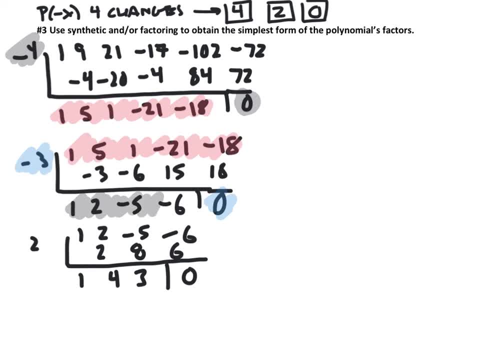 So then I have a new factor, this guy right here. I still am going to break this down one more time. I'm going to put it back into synthetic division and go at it with new numbers. Now again, I'm hitting it every time because I kind of know what's going on. 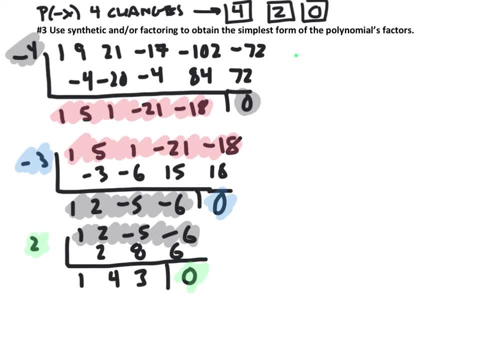 but you may miss sometimes and that's just a part of it. So I know that x plus 4 is a factor. because of this, I know, because of this, x plus 3 is a factor. Because of this, I know x plus 2 is a factor.